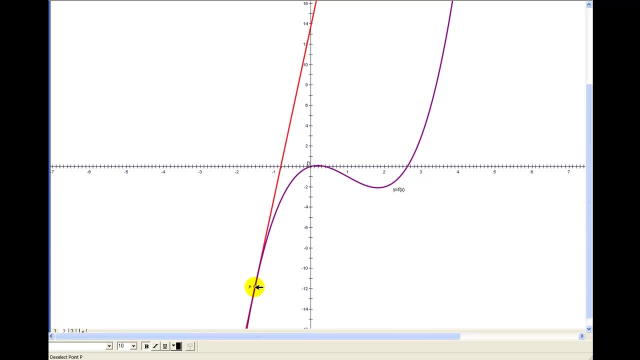 a positive slope, which is telling us that this graph is increasing or going uphill from left to right. As the slope of the tangent line remains positive, the derivative is positive and therefore the function is increasing As you reach this high point. at some point the derivative would be zero, and then it turns. 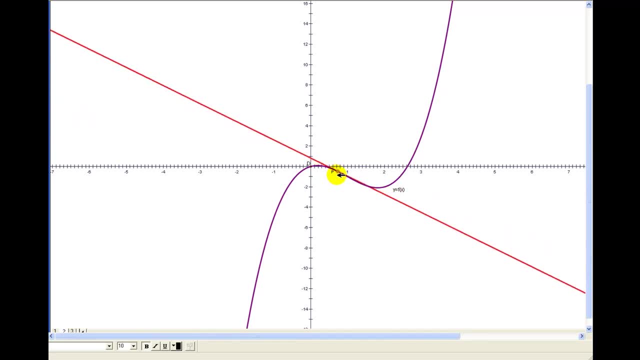 negative. If the derivative is negative or the slope of the tangent line is negative, the function would be decreasing on this interval. Somewhere around here the derivative is equal to zero, and then it turns positive again, so then the function again is increasing on this interval. 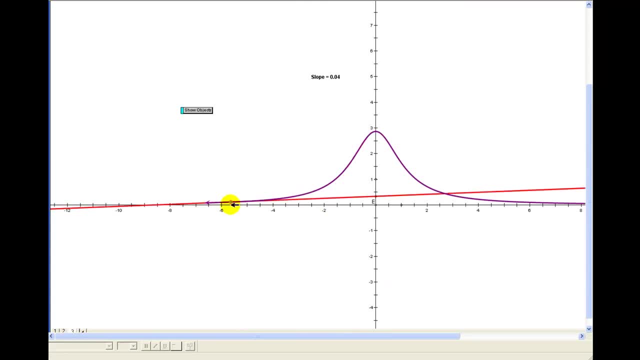 Let's take a look at another graph. Here we can see the slope of that tangent line is positive. therefore the derivative is positive and the function is increasing on this interval. It reaches a high point and then it turns to a negative slope, therefore a negative. 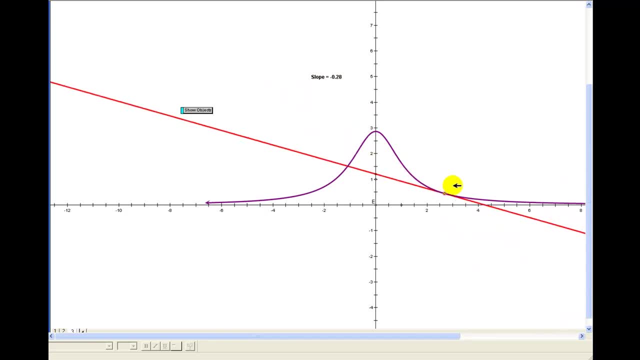 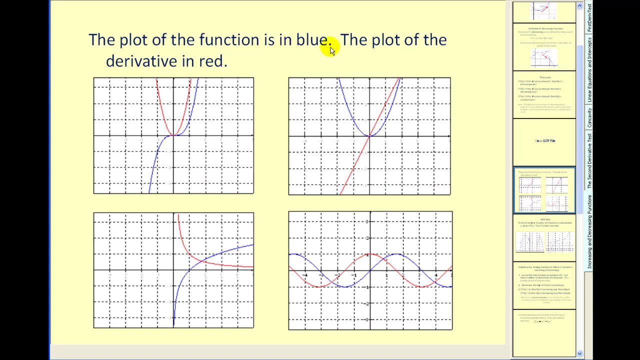 derivative and the function here would be decreasing because it's going downhill. Here's another way to look at the same idea. The plot of the original function is in blue and the plot of the derivative is in red. So if you take a look at the derivative function, 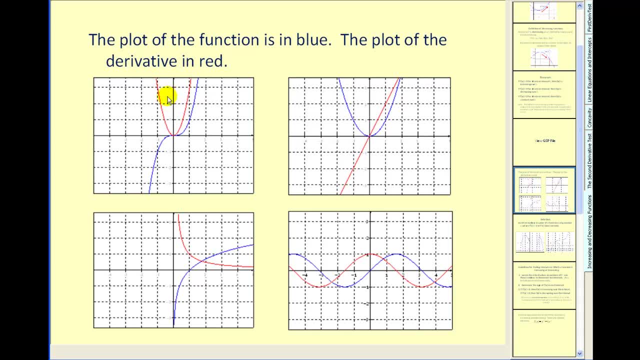 here in red these y values are positive. therefore the blue function is increasing on that interval. Here we can see the derivative would be zero and to the right of zero again the red function values are positive. therefore the blue function is increasing. This function is increasing. 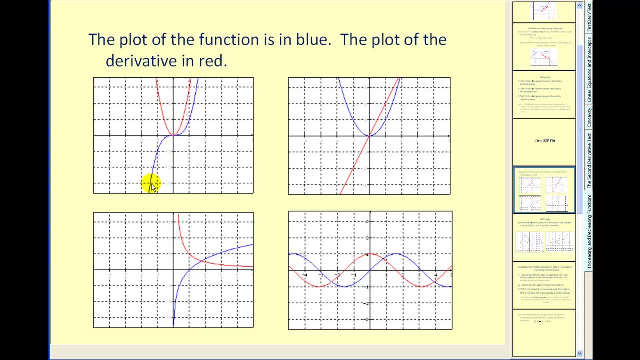 over its entire domain. so we call it a strictly monotonic function. Let's take a look at one more Again. our derivative is in red. so when we look at the values of the red function left of zero, they're all negative, which means the blue function should. 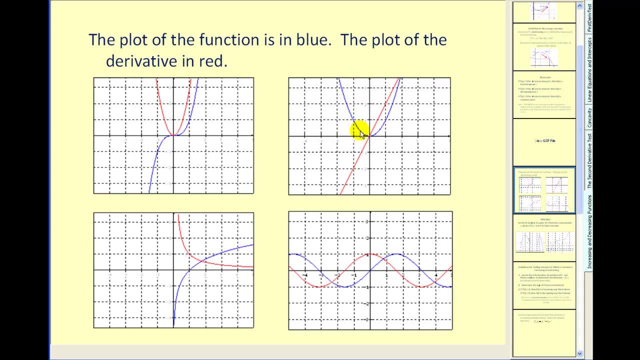 be decreasing, which it is going downhill. Then it's zero and then, to the right of zero, all of the values of the red function are positive. therefore, the blue function is increasing. You may want to pause and take a look at these other ones. I'm not going to discuss them due to time. This leads us to another important 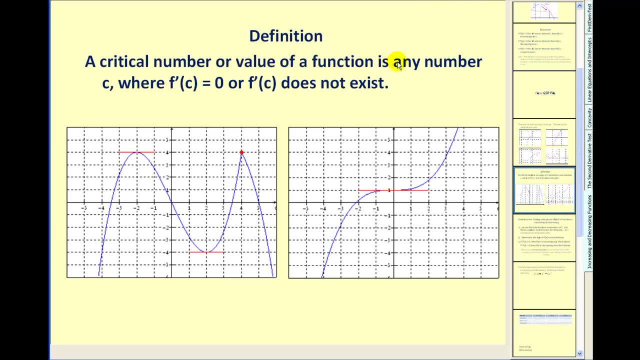 definition, A critical number or value of a function is any number- c, where the derivative evaluated at c is equal to zero or the derivative evaluated at c does not exist. It seems logical if we want to determine the value of a function, The first derivative we should find where it is equal to zero and then test to the 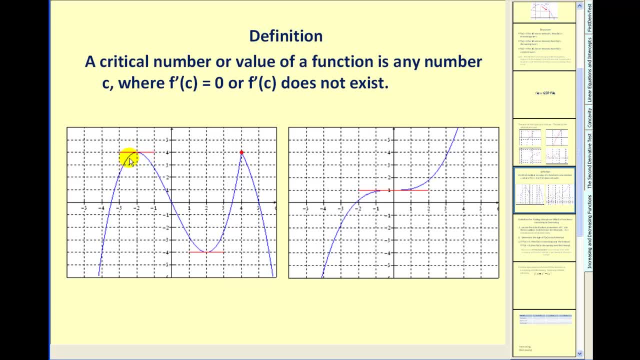 left and right of that value. Obviously, it will change signs to the left and right of where it is equal to zero. The derivative can also change signs here where the derivative does not exist because of the sharp point. We should note that just because the derivative 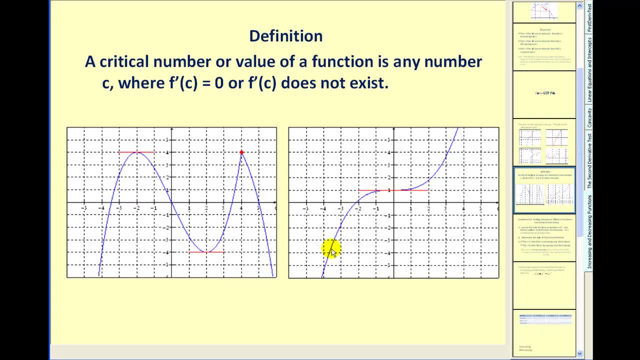 is equal to zero does not mean the sign of the derivative will change. We can see this function is increasing to the left of zero and also increasing to the right of zero. So here are the guidelines for finding intervals for which a function is increasing or decreasing. 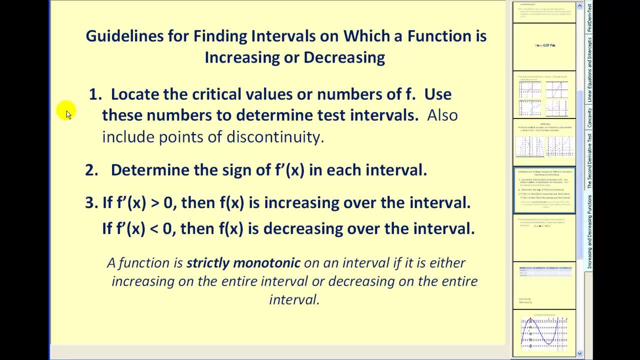 Step one, we're going to locate the critical values of the function. We'll use these numbers to determine the test intervals. We should also include points of discontinuity. Then we'll determine the sign of the first derivative in each interval and then we'll draw our conclusions. 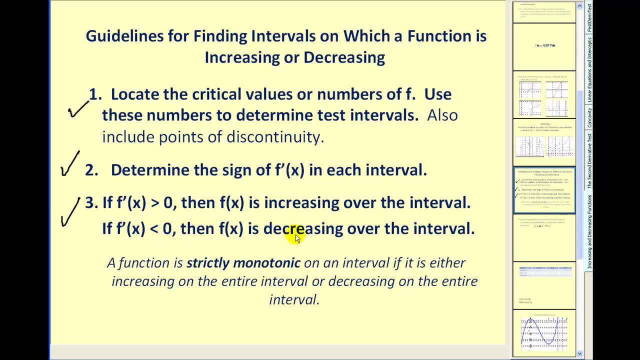 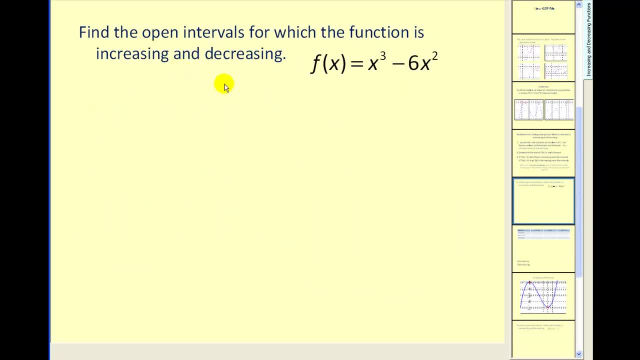 If it's positive, it's increasing, If it's negative, it's decreasing on the given interval. Our first example: find the open intervals for which the function is increasing and decreasing. So first we need to find the critical values or critical numbers, by finding the first derivative. 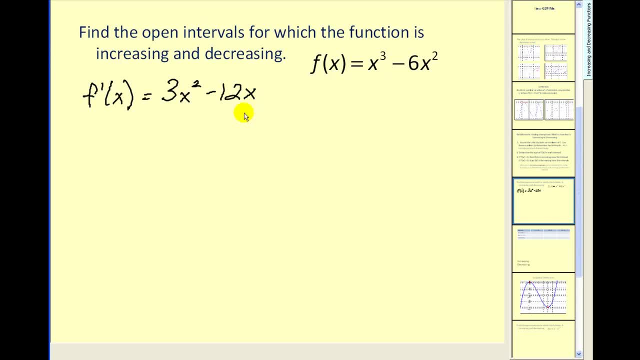 and determining where this does not exist or where it's equal to zero. There's no values of x for which this will not exist, so let's go ahead and set it equal to zero and solve. This is factorable. Looks like we have two critical values or critical numbers We have 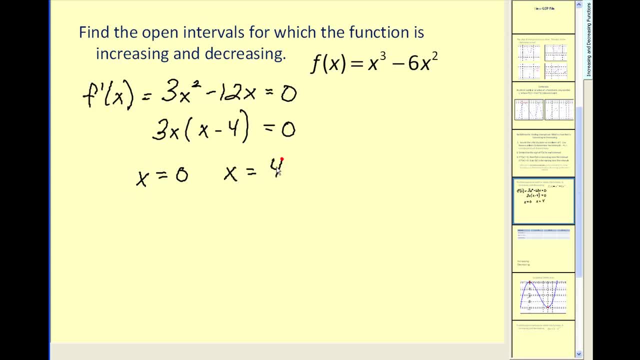 x equal to zero and x equal to four. Now these are the values we're going to use to determine our test intervals. Since the domain of the original function is all reals, if we want to determine on which intervals the first derivative is positive or negative: at zero it's equal to zero and at four it's. 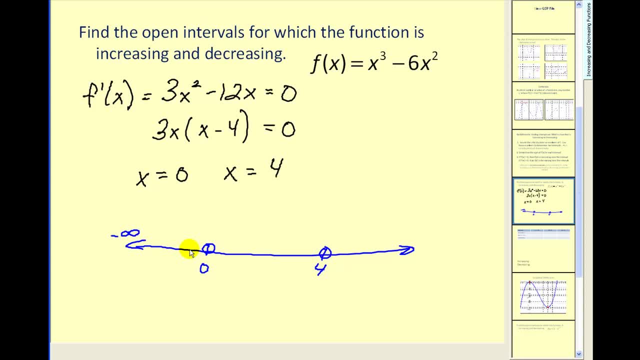 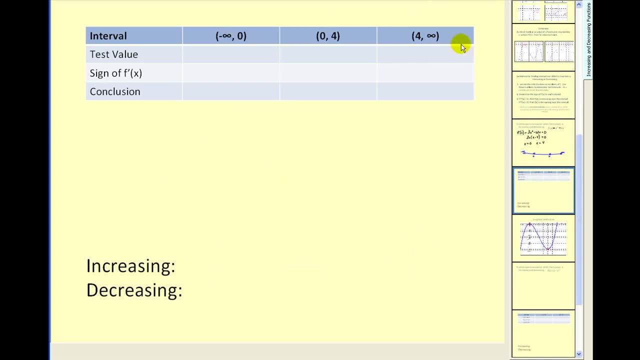 equal to zero. So we have to test the interval from negative infinity to zero, from zero to four and four to infinity. I've already set this up. Here are the intervals that we just discussed. Now let's pick a test value. We're going to use the interval x equal to. 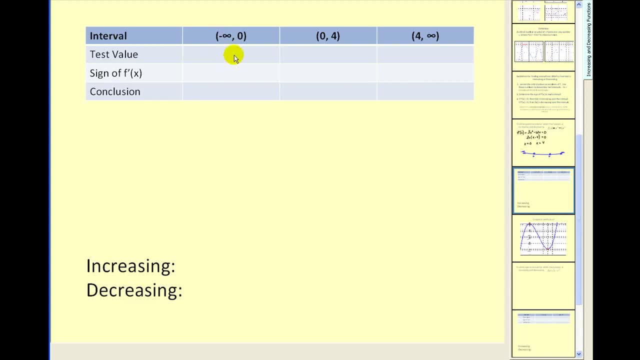 zero. We're going to put a value in each interval and determine the sign of the first derivative. So we can pick any value in here. Let's just choose negative one, maybe one and five. We are going to sub these values into the first derivative and determine the. 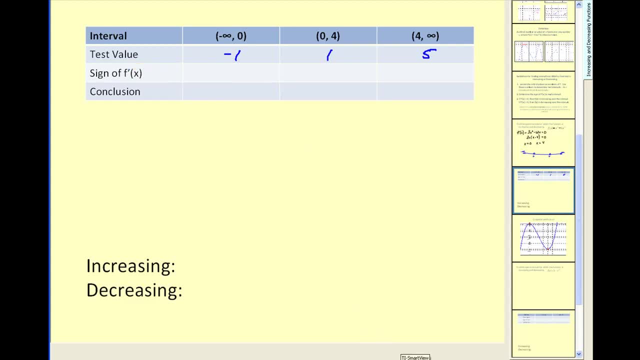 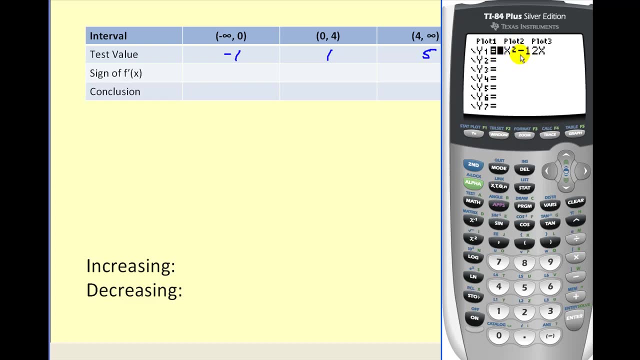 sign of the first derivative. Let's use the graphing calculator to do this. Now, I've already typed in the derivative function into y one. The derivative function was three x squared minus 12 x. To determine the sign at these given values, I'm going to use the table feature. 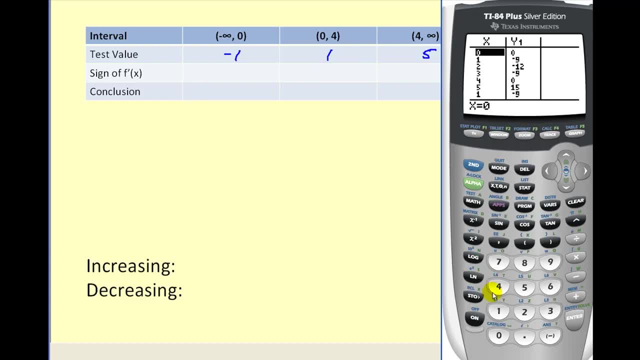 of the graphing calculator. Now, since my table is in ask mode, I can just type in: x equals negative, one, one and five. And again, I don't really care about the specific value, I just care about the sign. So it looks like the first interval is positive. 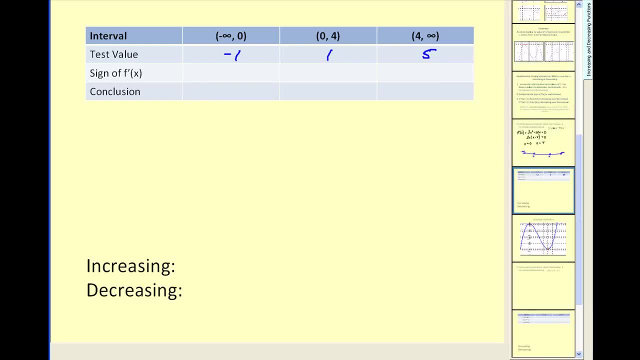 then negative, then positive. Let's go ahead and record this. So this interval is positive, this interval is a negative and this interval is positive. Well, we know, if the first derivative is positive at this test value, it's positive over this entire interval. 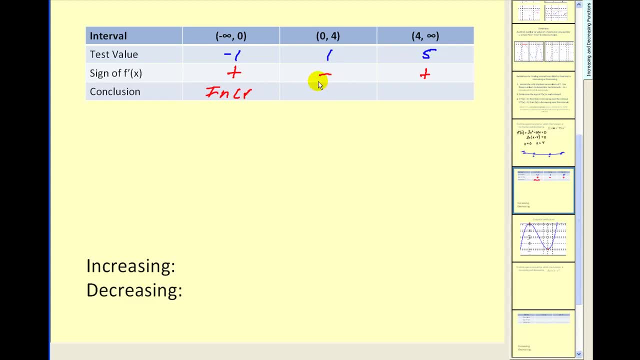 therefore it's increasing on this interval Because the derivative is negative here. it's decreasing on this interval and increasing on the remaining interval. So let's go ahead and summarize this down below. We know the function is increasing from negative infinity to zero. 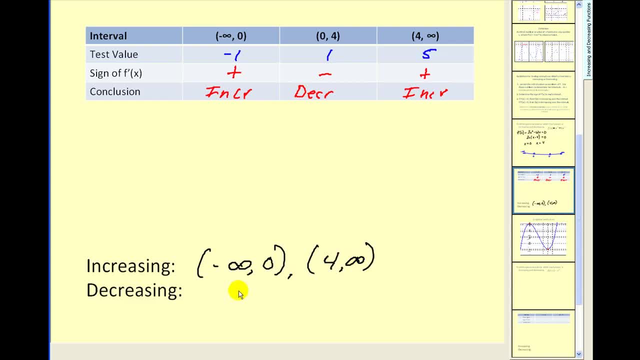 and also from four to infinity, and decreasing on the interval from zero to four. Let's take a look at the graph of the original function so we can verify what we have found. So, from negative infinity to zero, this function is going uphill. 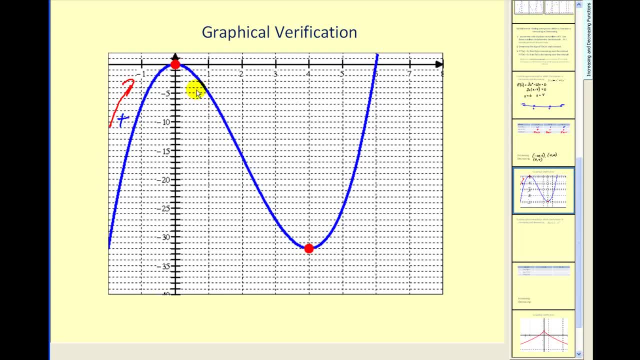 so it's increasing. where the first derivative is positive, From x equals zero to x equals four, it's going downhill or decreasing. So, as we found, our first derivative is negative, And then, lastly, from four to infinity, the function is going uphill. 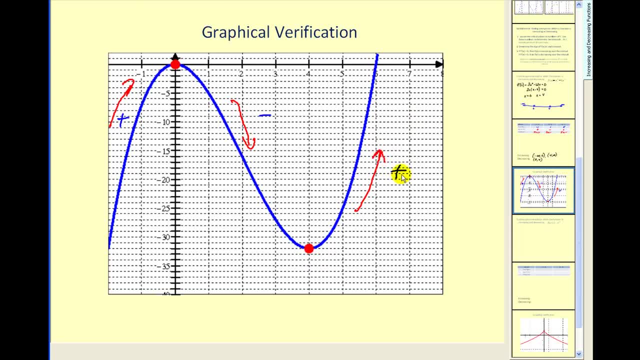 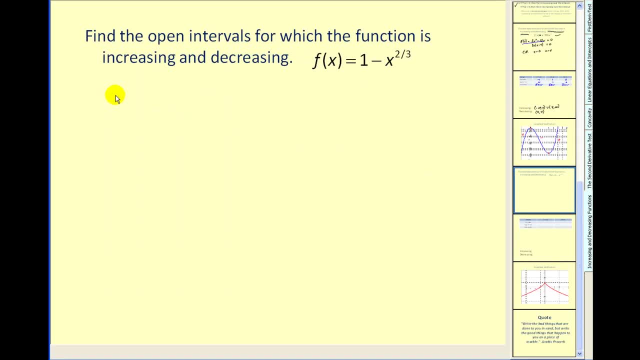 which verifies our first derivative should be positive, and in fact it was. Let's take a look at one more example Again. find the open intervals for which the function is increasing and decreasing. So we need to find the first derivative. So we need to find the first derivative. 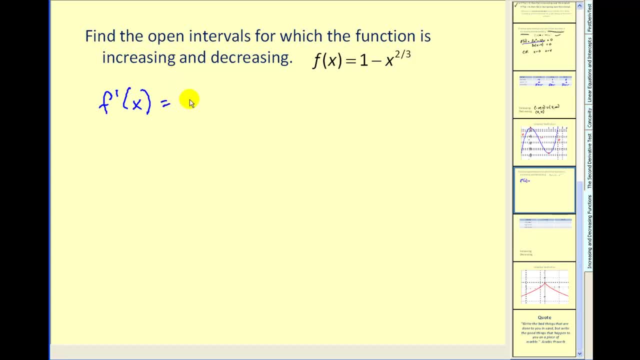 See where it does not exist or where it's equal to zero. The derivative would be equal to negative 2 3rds x to the 2 3rds minus one would be negative 1- 3rd. Simplifying, we'd move this to the denominator.